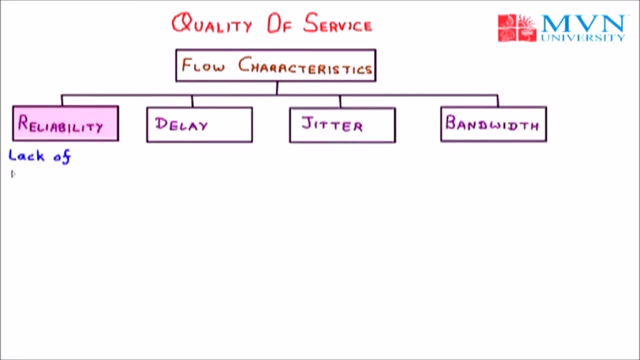 The lack of reliability means losing a package or acknowledgement Whenever any of the communication system lose the packet so many times. That means, for example, a source is sending the packet to the destination and there is loss. of packet. rate is very high. That means the reliability is very less. 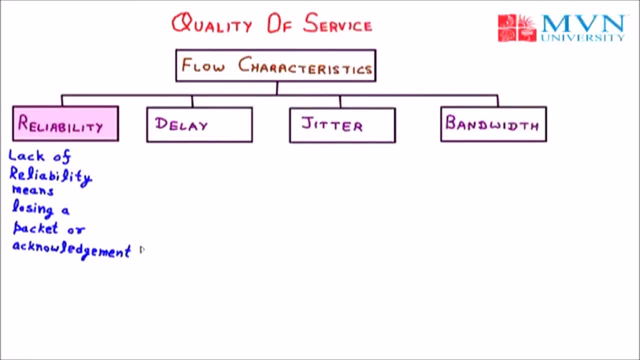 If the packet delivery rate is very high as well as the packet discarding rate is very low, That means the connection is reliable. And the next one is the delay From source to destination. the delay is the most important topic Because whenever we are sending the data from source to destination, how much time a packet will take? 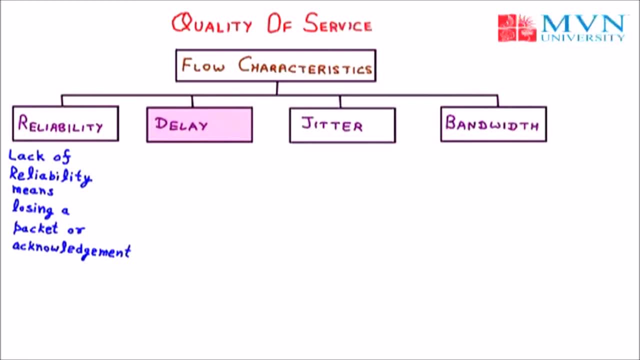 That is called the delay. If the delay is very high, that means the flow characteristics are not good, The connection is not good. But if the delay is very less, in that case the characteristics of flow are very high, The connection is very good. 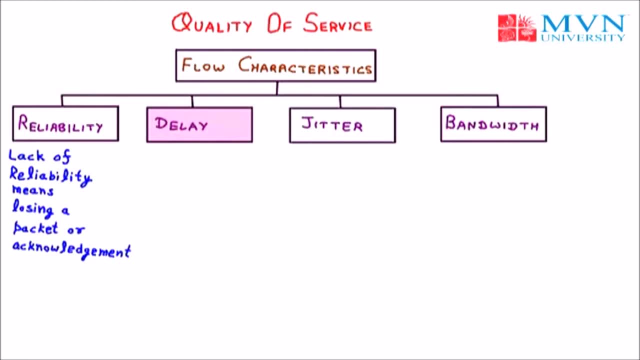 The application can tolerate delay in different, different degrees, For example, if I am talking about the high degree, Or if I am talking about the minimum delay required in applications like video conferencing or the audio conferencing or the remote login. So if I am talking about the delay, 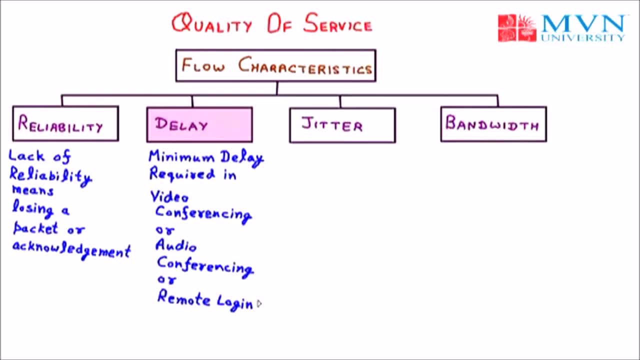 For example, we are doing the video conferencing. This video is streaming at the both parties from the source and destination. Both are in the conference. So in that case if we are having a small delay, That means the video will blur out, So the delay is required in very less amount. 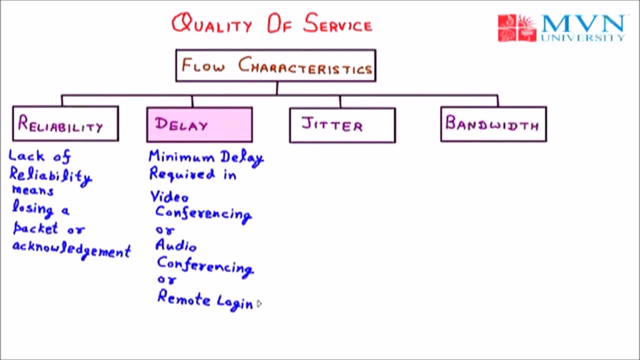 So that is why delay must be very less. If we talk about the audio conferencing, that is the same case as the video conferencing And obviously, if I am having the remote login, That means I am taking another system and my own system. 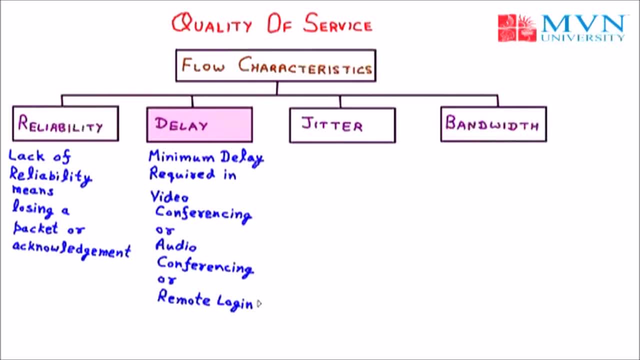 And in the remote login If I am just clicking on the mouse or any of the entry. in that case, If the action is not performed at the same time, In that case the connection is not good. So delay required is very less. So that is again a very important issue in the flow characteristics of the quality of service. 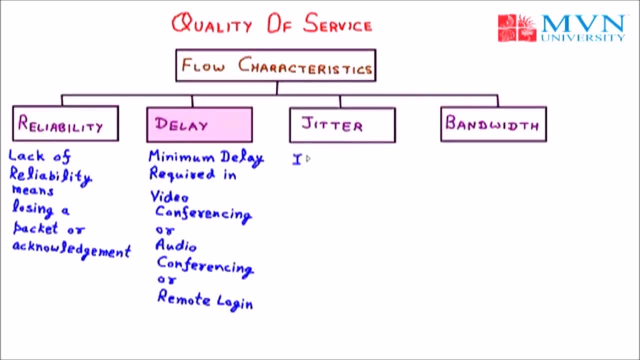 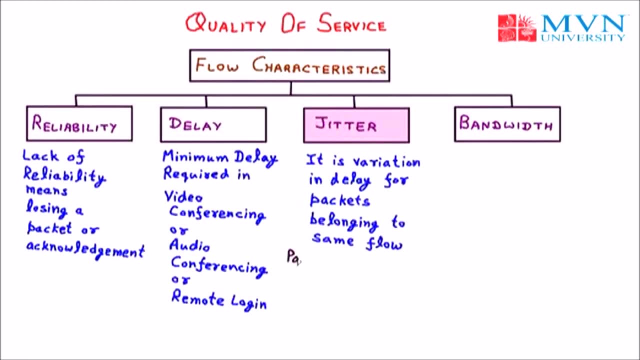 In the next one we are having a jitter. What is jitter? Jitter is basically the variation in delay for packets belonging to the same flow. Now we want to understand the jitter. Let us take an example of the packets. For example, we are having four packets. 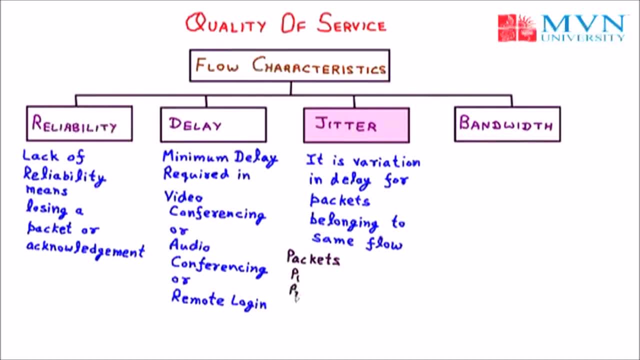 For example, P1, P2, P3 and P4.. Now we are having these four packets And let us suppose we are sending these packets at starting time. For example, the starting time of P1 is 0.. P2 is 1.. 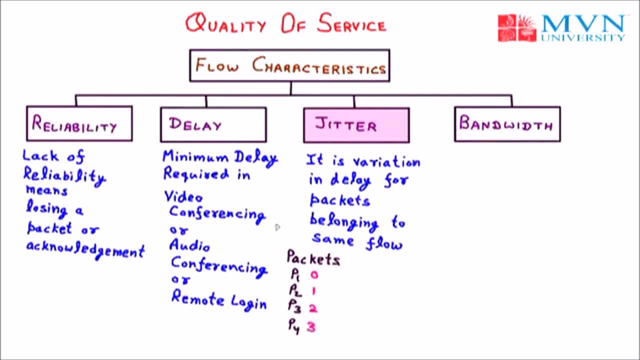 P3 is 2. And P4 is 3.. These packets received by destination. the time will be So let us suppose it is 20,, 21,, 22 and 23.. This is the particular receiving time of the packets. 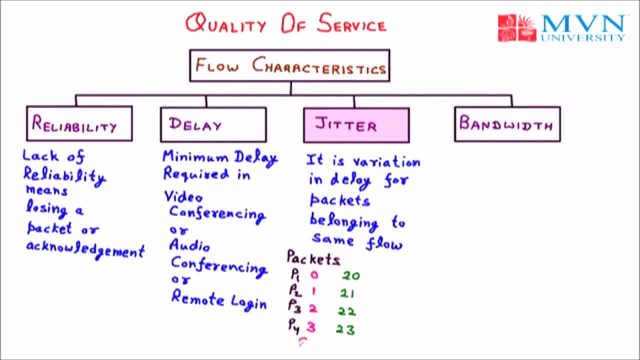 We are stating here as the ST as the sending time And the RT as the receiving time. So example: if I am going to call the delay, The delay will be 20 minus 0, that is equal to 20.. Again, 21 minus 1, that is equal to 0.. 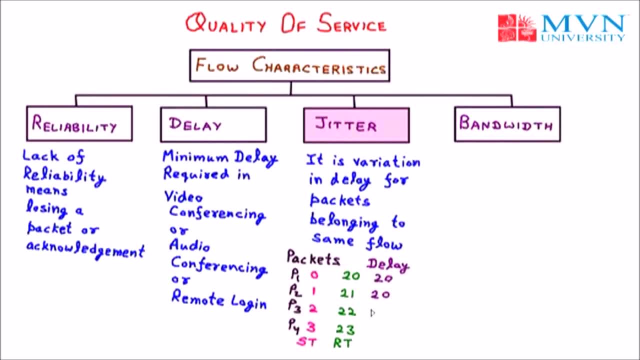 21 minus 1, that is equal to 20.. 22 minus 2, that is equal to 20.. 23 minus 3, that is equal to 20.. That means the delay is constant. that is equal to 20.. But let us suppose I am going to send the packet as 0,, 1,, 2 and 3 at the starting time. 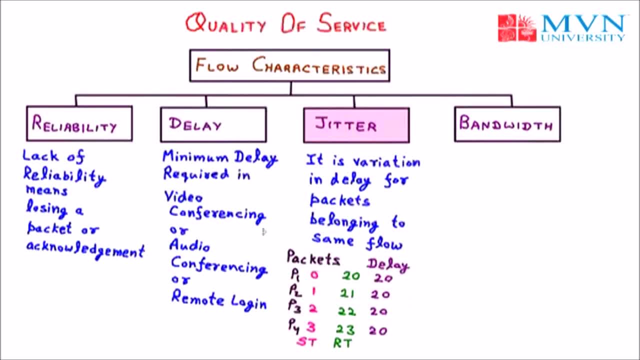 And let us suppose the receiving time is quite different. If we are having one more receiving time, That will be 21 for P1 and 23 for P2.. Again, 21 for P3 and 28 for P4. So these are the receiving time. 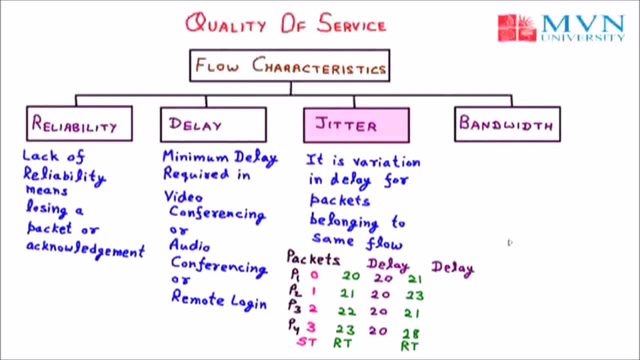 So in that case the delay will be quite different. So this is: 21 minus 0, that is equal to 21.. 23 minus 1, that is equal to 22. And 21 minus 2, that is equal to 19.. 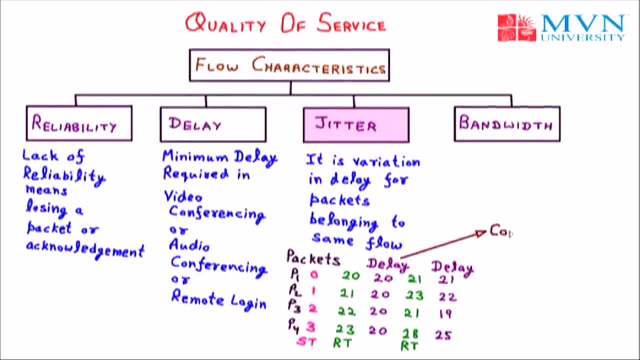 28 minus 3, that is equal to 25.. So we can conclude one thing: If I am talking about the post receiving time, We are having constant delay. The delay is constant. That means we can say that the jitter is very low. 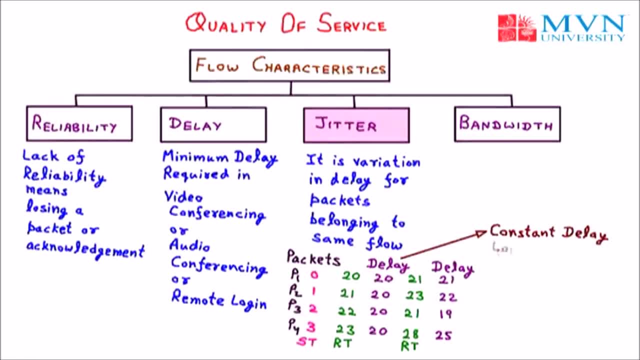 Because the difference between the sending and the receiving of the packet is very small. Then we can say that low jitter. And obviously the low jitter is required for the audio and video, Because if you have to send the particular audio and video, In that case the delay must be very less. 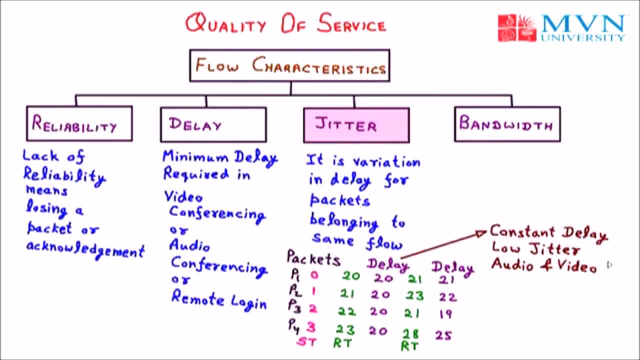 That means the jitter will be very less. The low jitter is required. But if I am talking about the second delay, The delay is very high. So we can say that it is the variable delay. As we are having the variable delay, That means the delay is very high. 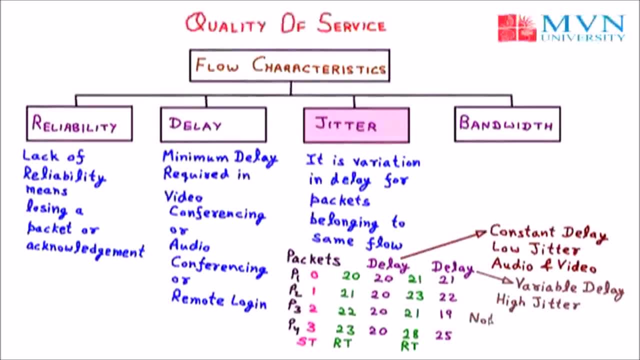 So we can say the high jitter And the high jitter is not acceptable And not suitable for audio and video. That means for sending the audio and the video file We need to set the low jitter And for low jitter we need a good connection. 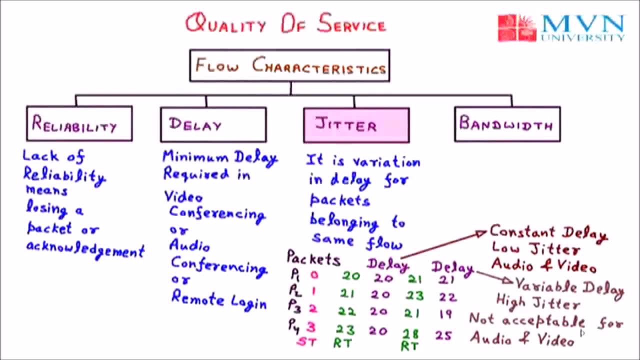 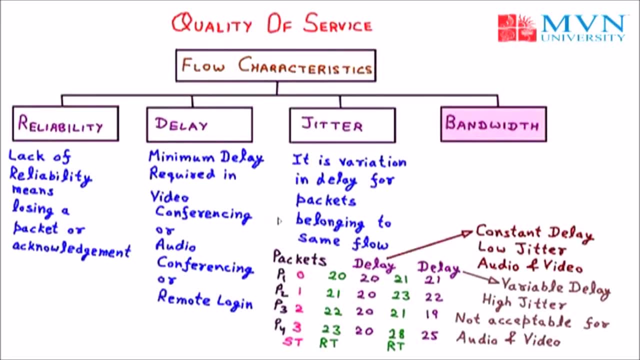 And good connection. That means the constant delay is required. Now the next one. we are having The bandwidth and the flow characteristics of quality of service. The bandwidth is required for sending of the data. That means, for example, we want to send the data from source to destination. 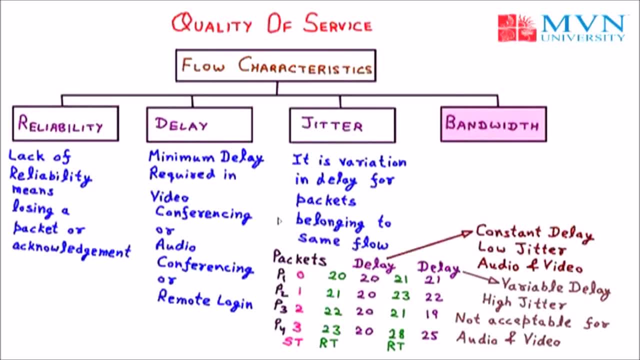 The bandwidth is required. That bandwidth is all about the sending of data Or the speed of data. Different application need different bandwidth. For example, if I am talking about the high bandwidth That is required for video conference, If I am talking about normal email, 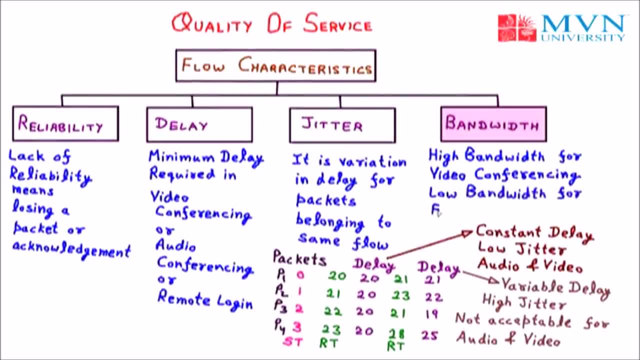 The low bandwidth is required. So we can say that the low bandwidth is required for sending an email, Because in the email we are having the low data. We have to send only the text file Or maybe the video Or the small pictures. 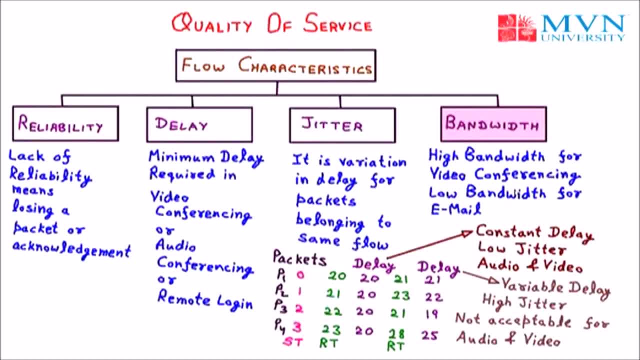 So in that case the bandwidth- That means the speed of data connection- is very less, So the low bandwidth is required. I am talking about the video conferencing. We have to send the synchronized of data Video and the audio. In that case, what we need 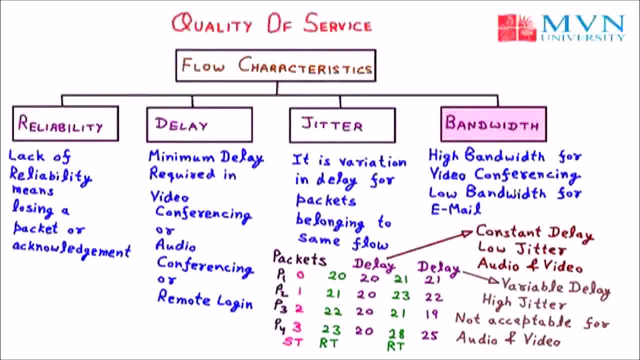 The high data rate. High connection, That means high speed. That is all about the high bandwidth. So bandwidth is the most important flow characteristics of quality of service. So we have discussed about the four flow characteristics. That is the reliability. That means how much connection is reliable. 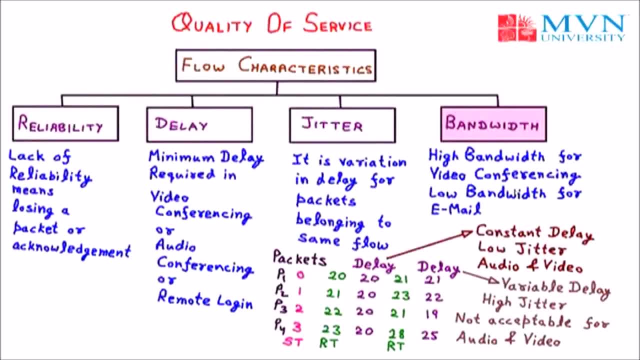 Then the delay. That means the sending and receiving of data. We are having some delay. Then the jitter, The variation in the delay, And the bandwidth, The speed requirement. Now we will discuss the techniques to improve the quality of service With the help of these flow characteristics. 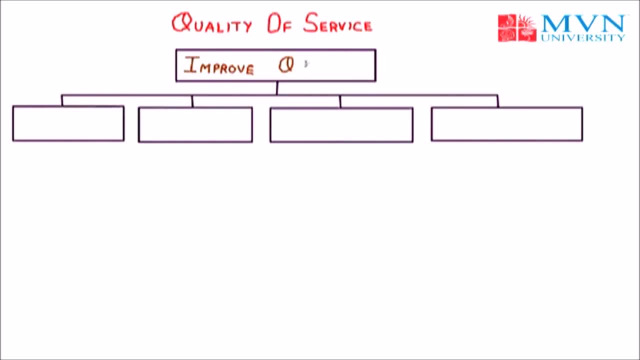 Now we have to improve the quality of service. It gives a stamp on the quality of service. Then we are having the four steps. That is scheduling, Next is traffic shaping, Next is resource reservation And the last is admission control. Now the improving quality of service. 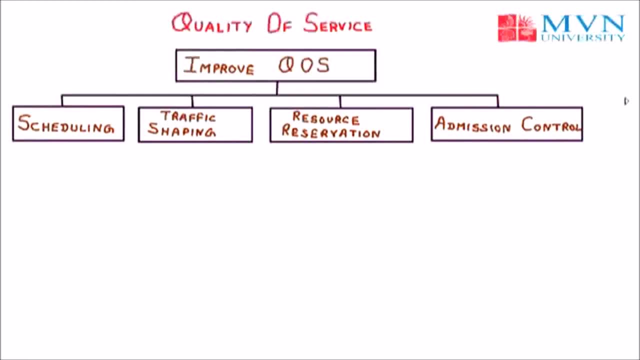 That means we have to improve the quality of service. We are having the fourth step, That is, the scheduling. If I am talking about the scheduling, The packets from different flows arrive at the switch or the router for processing. A good switching technique creates the different flow in a fair and appropriate manner. 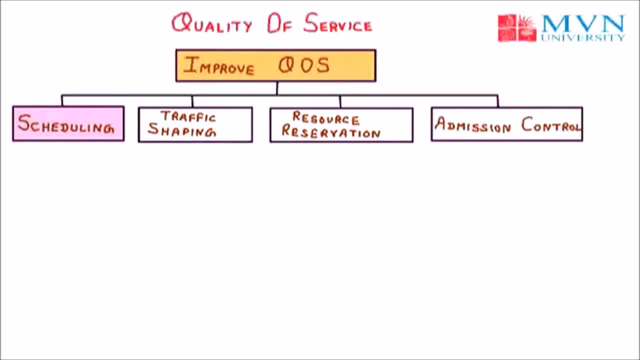 Several scheduling techniques are designed to improve the quality of service. The first scheduling technique we are having, That is the FIFO queuing, The next thing being into the scheduling we are having, That is the priority queuing, And the next into the scheduling we are having. 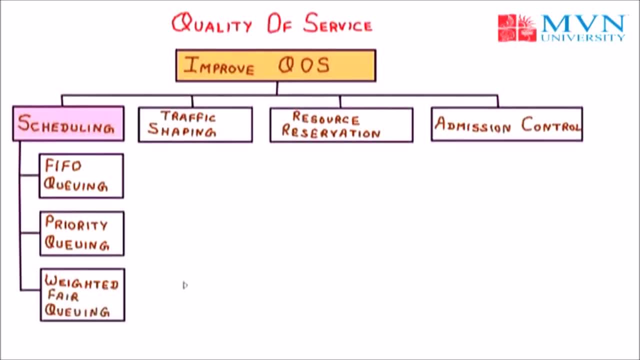 That is the waiting queueing. So first of all in the scheduling we will discuss the FIFO queuing. Under the FIFO we are having the FIFO That is called the first in, first out queuing. For example, we are having some particular packet. 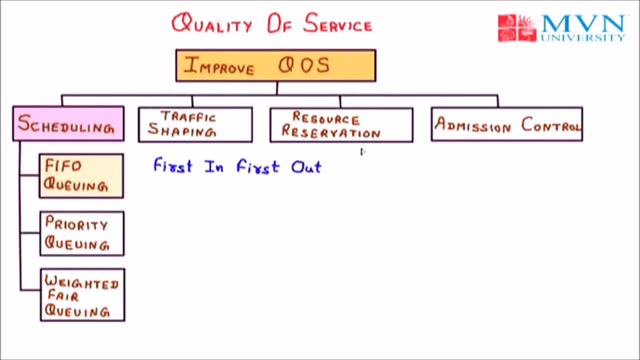 That is received by the destination first or the router first, Then it will serve that packet first in. To understand FIFO queuing, or the first in first out queuing, So first in, first out queuing. Let us take the example of the diagram. 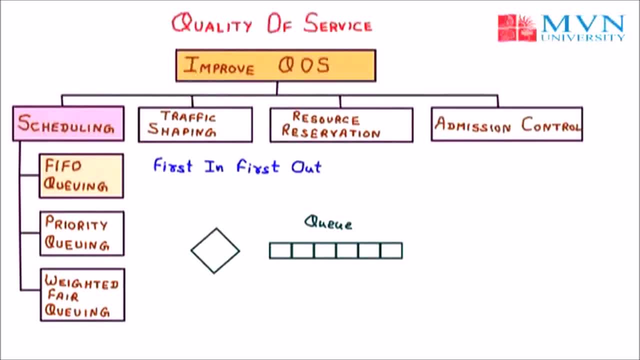 Let us suppose we are having queue. Let us suppose we are having some packet. First of all, packet will be arrived in the decision box. The decision box will check whether the queue is full or not. Let us take the example of the queue. 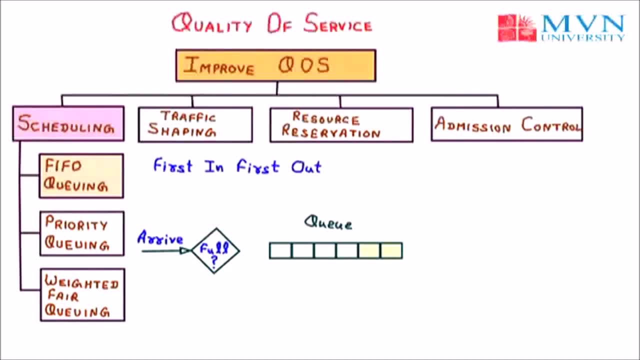 We are having the two entries which are filled. That means the queue is empty. It is not completely filled. In that case the packet will be sent to the queue. But let us suppose the queue is full. In that case it will discard the packet. 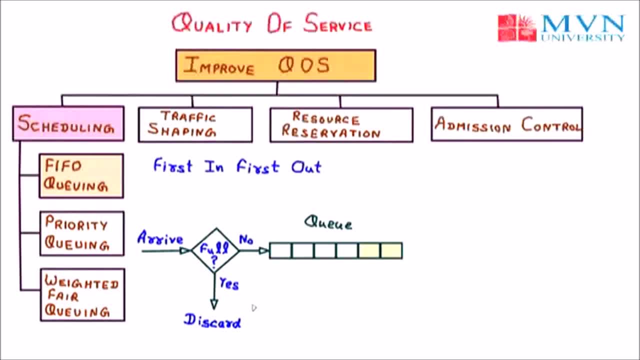 Now the packet will be sent to the queue And queue will take that particular packet at the back side, exactly after the two packets. So after the queue, we are having a processor in the FIFO queuing, So the packet is sent to the processor. 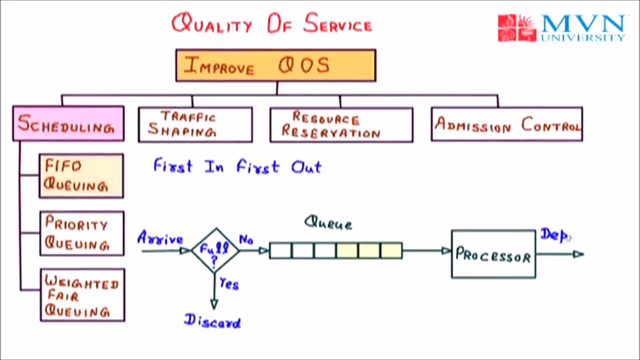 And the processor will process the packet And will then send for the departure, So that we can say that this is the first come, first serve. That is the FIFO: First in, first out, And that means the packet is arrived in the queue. 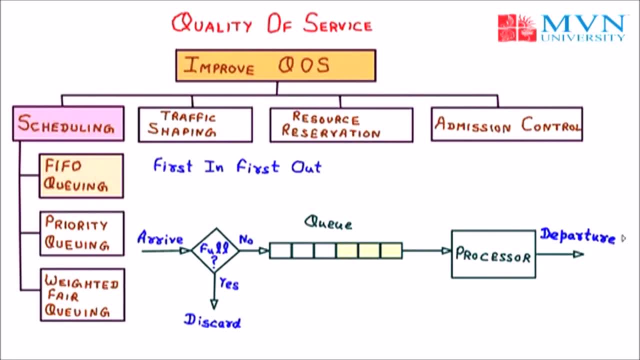 And is processed And is sent out. Next we are having that is, the priority queue. In priority queuing, packets are first assigned to a priority class. Each priority class has its own queue. The packets in the high priority queue are processed first. 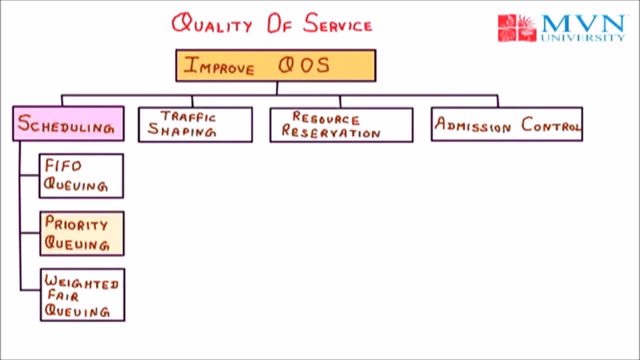 Packets in the low priority queue are processed last. So to understand the priority queue, let us take the example of the diagram. Suppose we are having two queues. We can say that the first queue, that is the high priority queue, And the second one is the low priority queue. 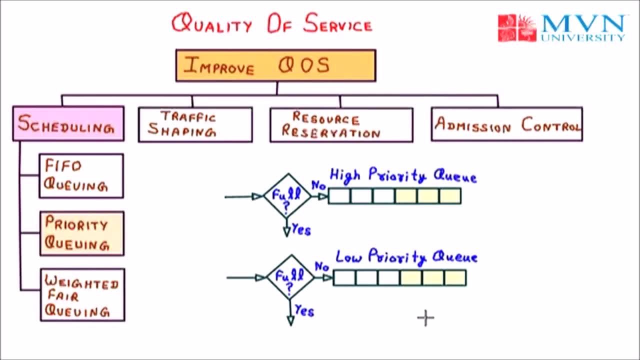 Before the queue: we are having the same decision box as we have already discussed. We will check out whether the queue is full or not. First of all, the data packets will arise And they will be sent to the classifier. After the arrival of data packets: 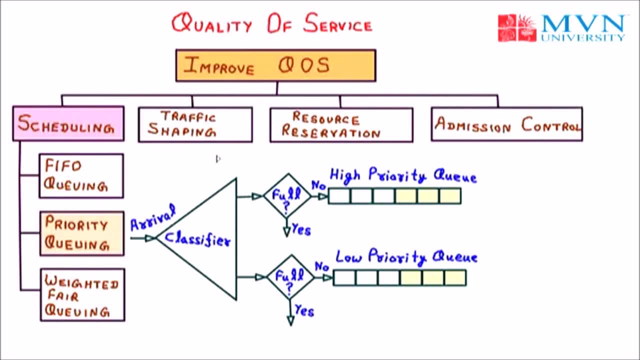 The classifier will take those data packets And divide the data packet accordingly. For example, data packet is of high priority, It will send the packets to the high priority queue And the packet is of low priority, It will send it to the low priority queue. 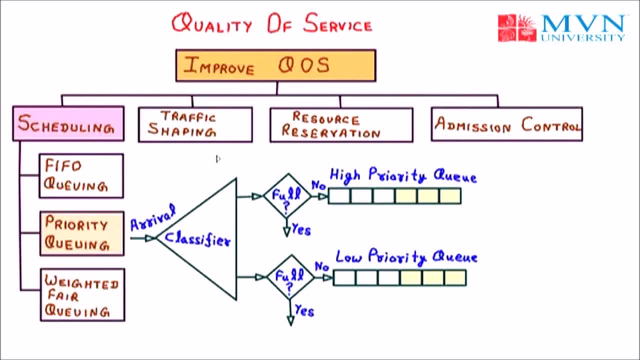 Then, after the priority queue, We are having the processor. The processor is having a switch That will be connected to the both ends of high priority and low priority queue, But one at a time. At the both ends of the queue we are having a particular button. 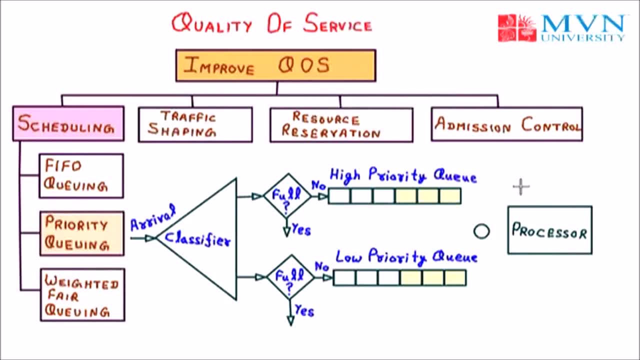 To which the queue will be connected, And the switch will connect to that particular button Here Which will send the data to the particular processor. Now let us suppose we are having the packet. The packet will be arrived to the classifier. The classifier detects that the packet is of high priority. 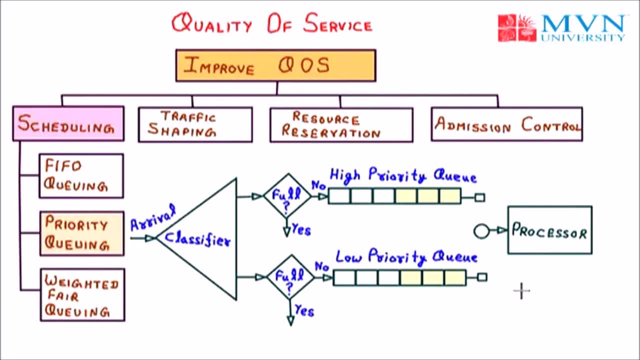 It will check out whether the queue is full or not. If the queue is not full, It will send the packet to the high priority queue And after the high priority Processor will come to know the packet is coming from the high priority, Then the processor will indicate to high priority queue. 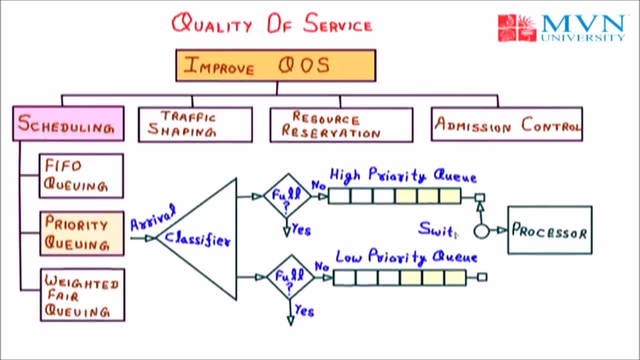 And the switch will take the packet from the high priority queue. Now, whenever the queue is full, The switch will be switched to another queue, From the high priority to the low priority. Now the processor will take the data packet From the switch of the high priority. 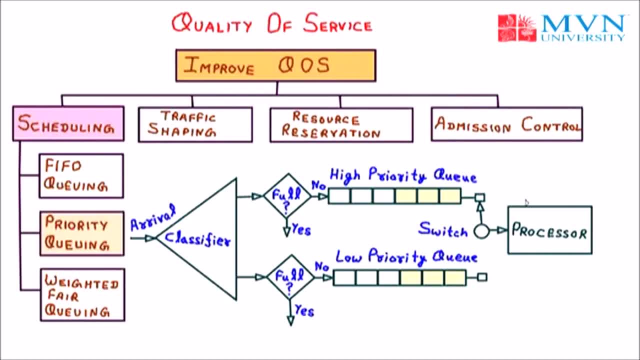 And it will send the data packet outside For the departure. So that is all about the priority queueing, In which we have assigned the priority With the help of the classifier. Next we are having the weighted thread queueing. Now the batter should look like this: 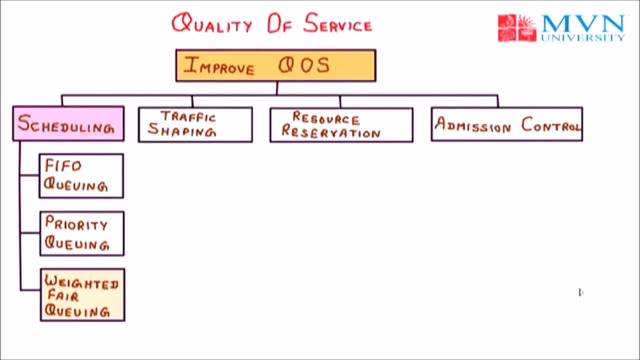 The weighted thread queueing method is the weighted thread queueing. In this technique, The packets are still assigned to different classes And are admitted to different queues. The queues, however, Are lifted Based on the priority of the queue- Maybe the higher priority? 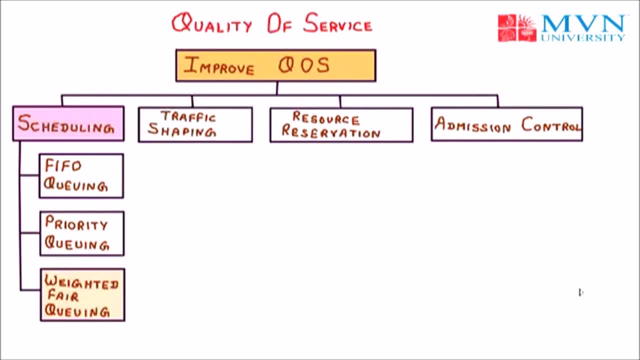 Higher priority means higher weight. The system processes packets In each queue In a round or big fraction, With the number of packets Selected from each queue Based on the corresponding weight. To understand the weighted queue, Let us take an example. 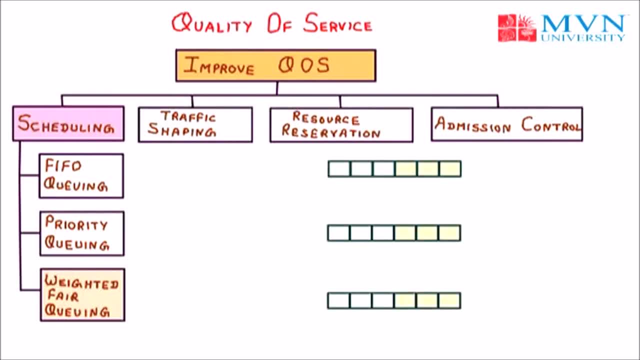 In which we are having Three queues. These are the three queues. Where will we assign the weight To all the queues? Because this is the weighted thread queueing The first queue. We will assign the weight as the three. The second queue: 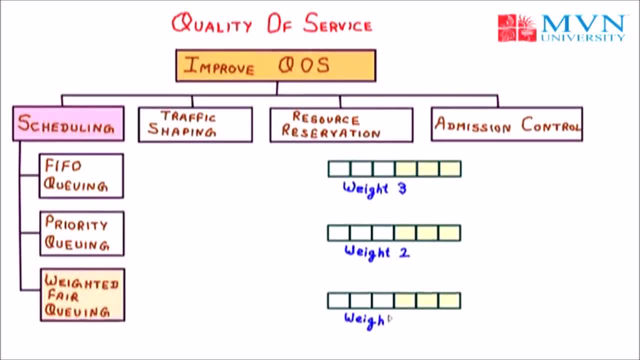 The weight is two. To the third queue, The weight is one. Now all these three queues Have the decision box as the prefix For the decision boxes. We are having the classifier. After the queues, We are having the processor As well as the switch. 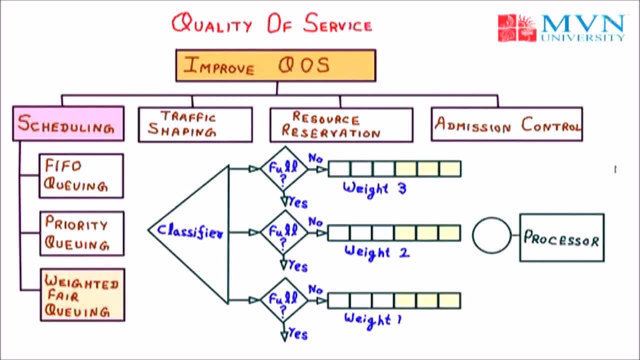 The switch is connected with the processor. All the three queues are connected With the switch. Now let us suppose There is an arrival of the first packet. It is sent to the classifier. Now, when the packet is arrived to the classifier, The classifier will send. 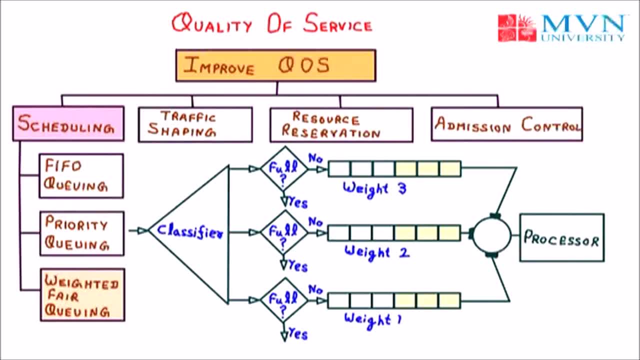 The packet to the particular queue. Now we are having the three queues, Having the weight three, Weight two Or weight one. Now If the queue is supposed to start the packet, Otherwise, The packet is sent to the particular queue. Let us suppose the packet is sent. 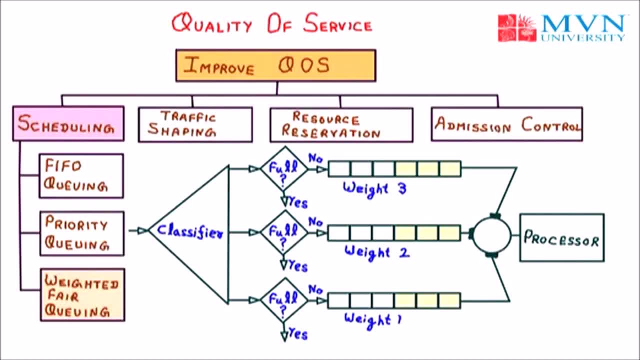 To the weight three. Now In the processor We are having the switch Switch is connected to all the queues. Now The switch is rotatory, Now the switch is connected to all the queues And the processor, The switch, is rotatory in the clockwise direction. 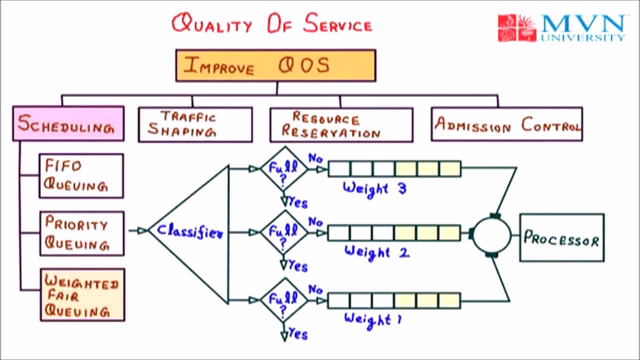 The direction And the connectivity of switch Is first assigned with the weight three queue. Now the switch direction can be Rotated From Weight three, Weight two To weight one In the clock, Or the other way around. So 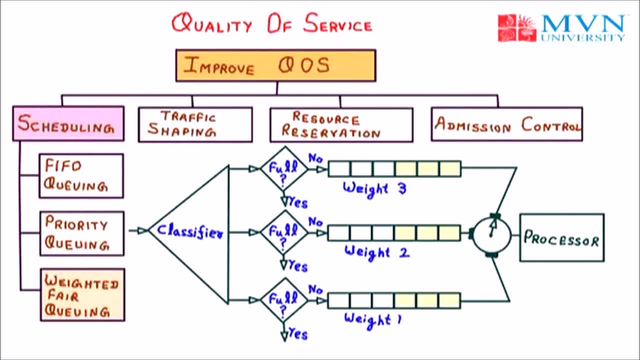 The weight three, The weight two, The weight three, The weight one And the clock In the clock Or the anti-clockwise direction. Let us suppose The switch is first connected To the Weight three. That means It will take. 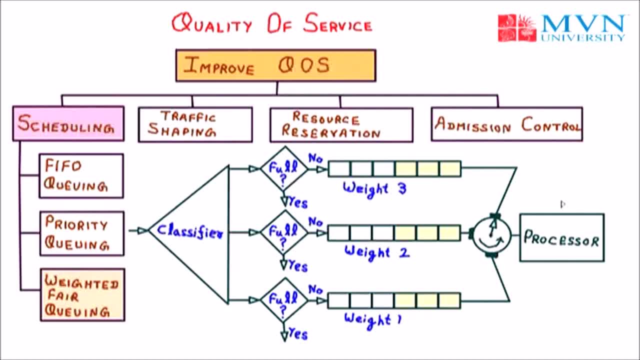 Three packets From the queue one. Now It will pass to the processor And the packets will be Departure out. If the direction of switch Is set to The queue number one, That is, for weight three, Then it will take. 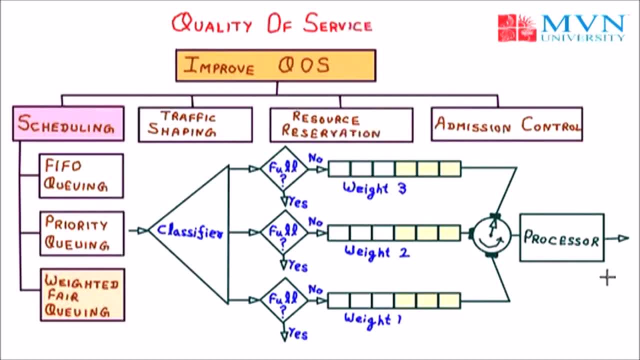 The three packets And process them. Next It will check out The weight two Queue And it will take The two packets From the two queue. Then It will Next To come to the Queue three. It will take 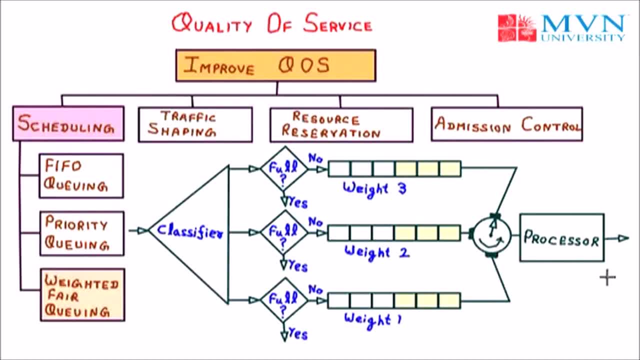 A single packet Because The weight assigned Is one. So that means If the weight is three, It will take Three packets. For the weight is two, It will take Two packets. For the weight is one, It will take. 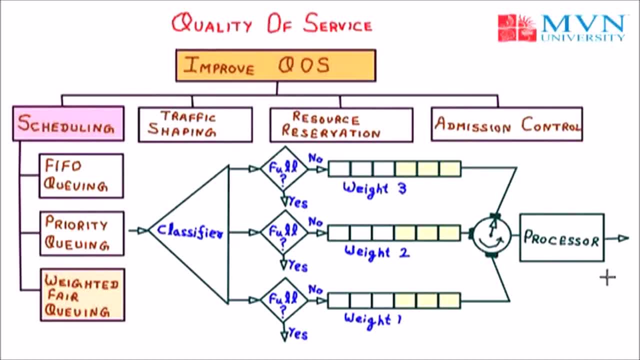 One packet. So that is all about The weighted fair queue, In which The packets are based upon Their weight. They will depart The packet According to their weight. Now We will discuss The next Quality of service. 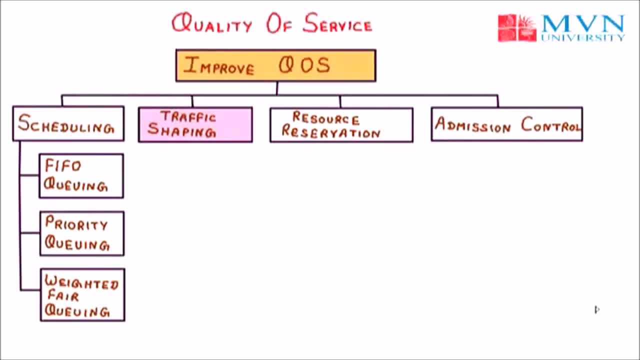 We will discuss The amount And the rate Of the traffic Sent to the network. Basically, We are having Two types Of traffic Shaping techniques. The first one is The leaky Bucket. The next technique. 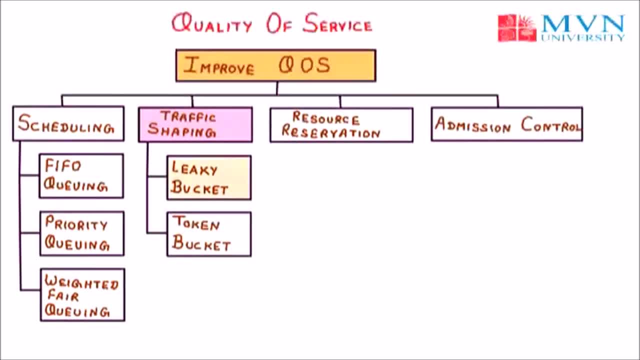 We have Is the Token bucket. So First of all We will discuss The leaky bucket. Well, The leaky bucket Algorithm Shapes Bursty traffic Into Fixed Size. Let us Take the example. 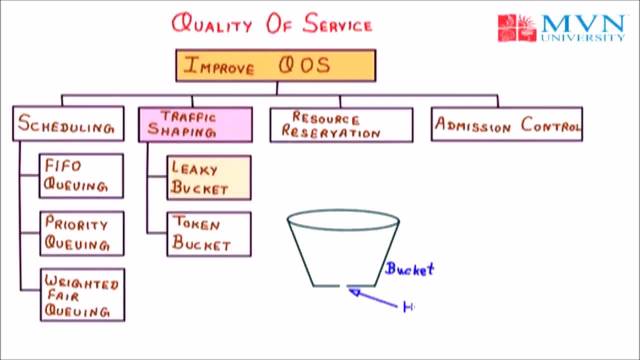 Of the diagram. Now Let us Suppose We are having A bucket. In the bucket And the button We are having A hole. Now Let us Suppose We are having A tap That is Over the bucket. 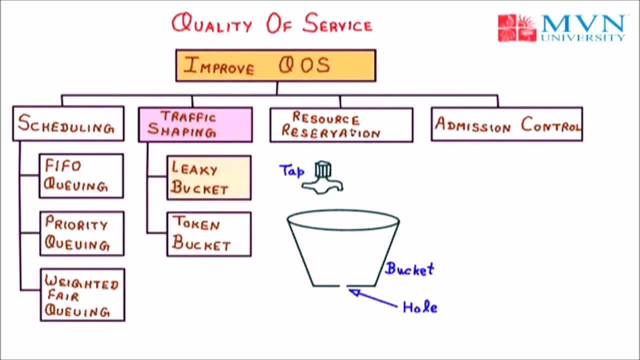 Now This tap Will spread The bursty data. Bursty data: That means There is A no particular Sequence Or the variable, So It is the bursty flow of water. Now That water will be. 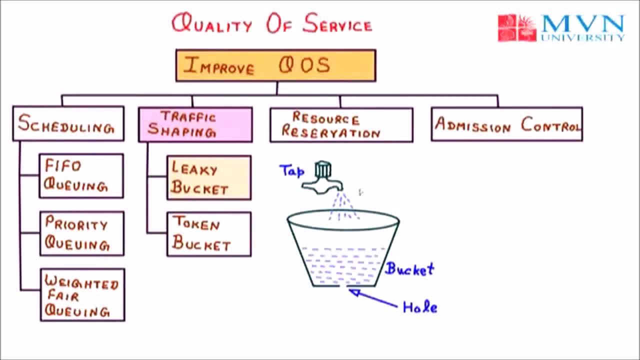 Collected Inside the bucket. So This is the bursty data Or the bursty water. So We call it as The bursty flow of data, As you can see that At the bottom There is a hole. 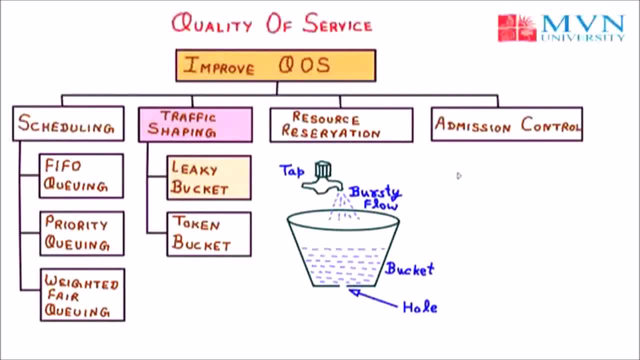 In the bucket. That means There will be Water which will come out From the hole. There is a main And a major point To be noted: That from the hole The data will come out, But the water will come out. 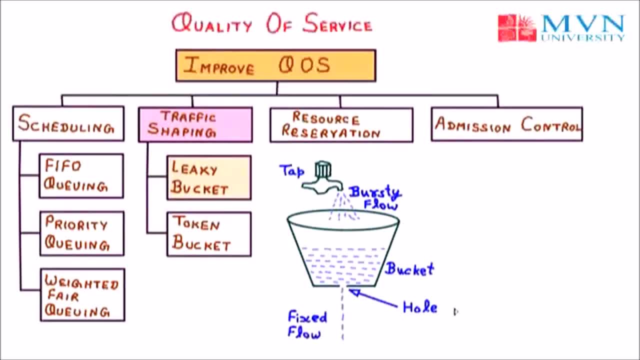 That means That will be of Constant flow. We can say that With the help Of the leaky bucket, The bursty flow Of data Or the water Can be converted to The fixed flow Of data Or the water. 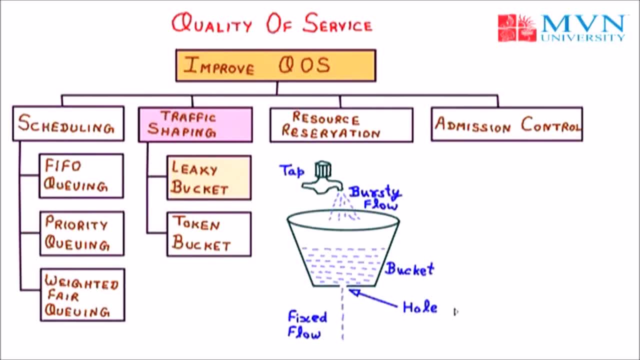 Now, Compared with that, We are talking terms, See example. We can say The data And the bursty form. Let us draw A graph For that. Suppose We are having A timeline On the x axis. 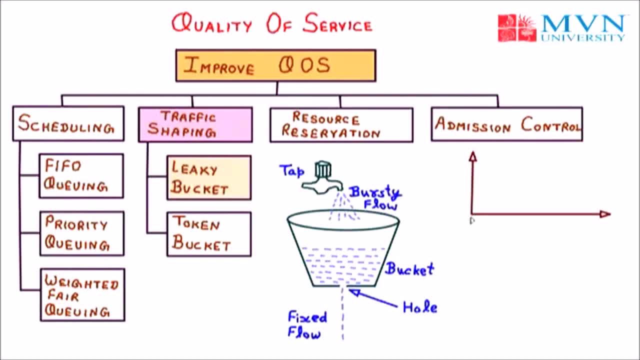 And the data rate On the y axis. I am going to divide The timeline Into 10 particular parts, Starting From 3. 4., 5., 6., 7., 8., 9., 10.. 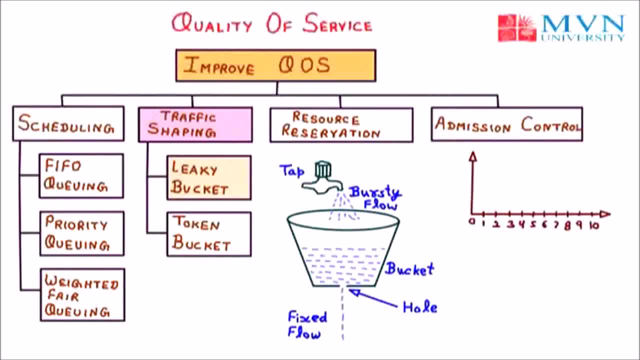 Now Let us suppose For first 2 unit of second We are having 12 MB of data, So Data rate will become 12 MBPS. Now Suppose For the next Few seconds. System is ideal. 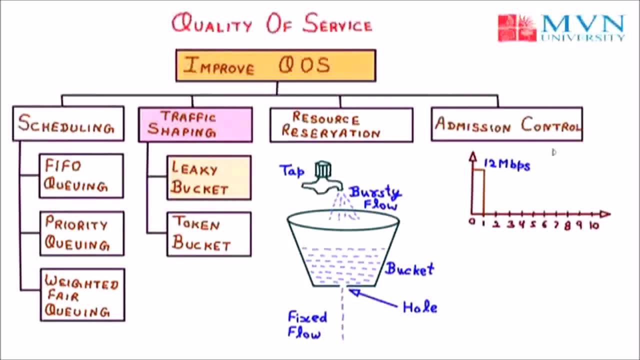 And after that From 7 to 10.. We are having 2 MB of data. So 2 MB of data That means For the first Second We are having Data of 12 MB, That is. 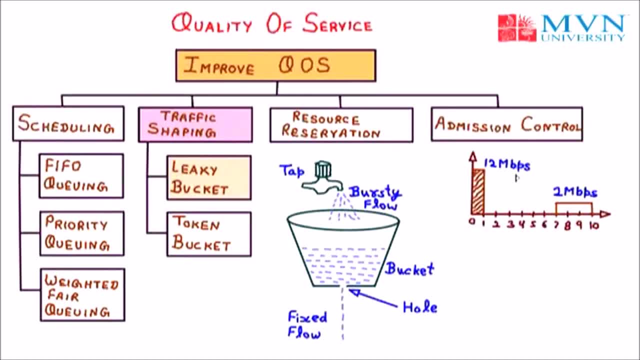 12 MBPS And for the Next few seconds The data rate is Ideal And after The next 3 seconds We are having 2 MBPS of data, So We can also State that That is. 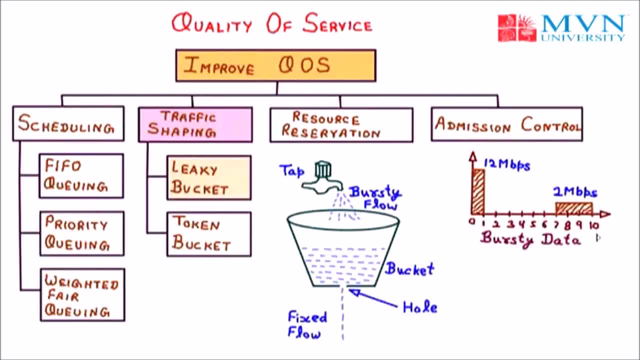 This is the Bursty form of data. We can also Consider as the Bursty data. Now Compare it With the Leaky bucket. The sum time Flow is ideal. And now again For the sum time. 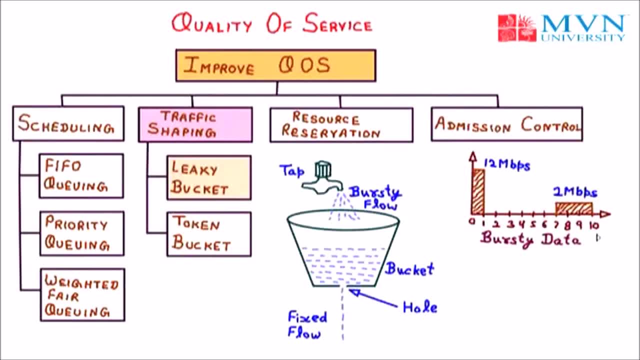 The flow become Very low: 12 MBPS. 0.. 2 MBPS- Same in the graph. Now, As we follow the Leaky bucket algorithm, The data must be of Fixed flow. So that means If we count. 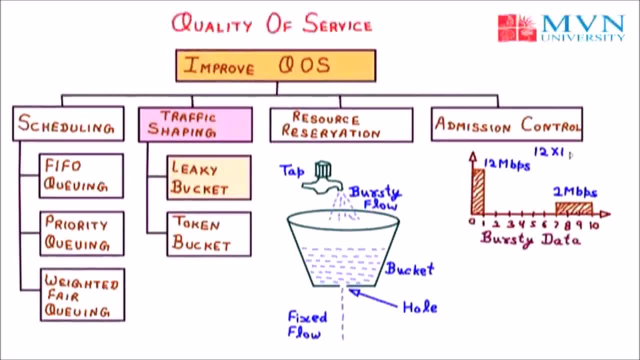 The complete data rate. The complete data rate is 12 into 1.. That is 12. Plus 2 into 3. That is Equivalent to 12. Plus 6. That is Equivalent to. 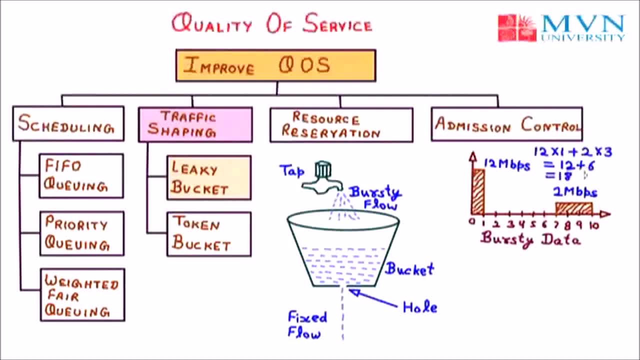 18. That means In total, We are having 18. MBPS Of Data. Now, Whenever we find out The fixed flow After The leaky bucket, We will modify The diagram Of the graph. 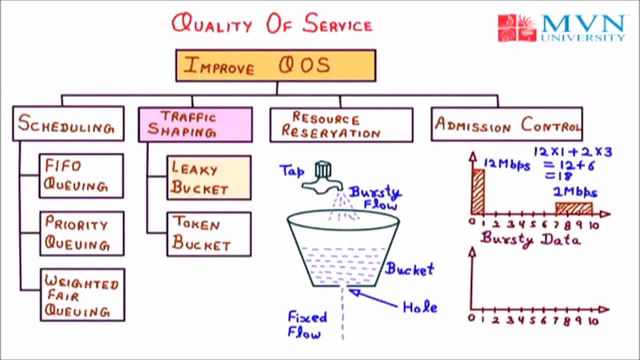 Now Let us suppose We are having The complete data, That is, The fixed flow data, That is, of 1., 8. MBPS For the whole 10 seconds. So We can say that 1.. 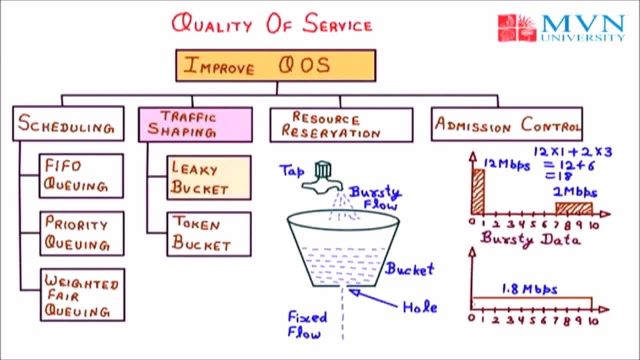 8. MB For the whole 10 seconds. So We can say that 1., 8. 10. Is equal to 18 MB Of Data, So We can say that It is the 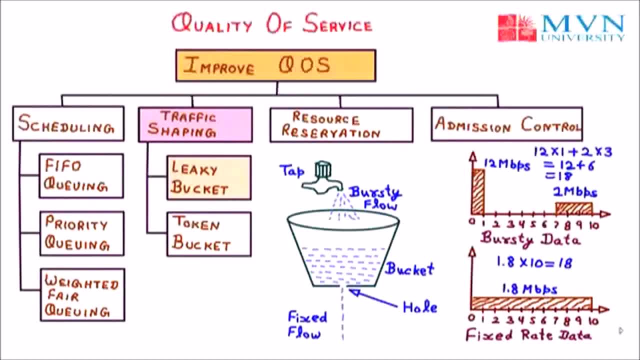 Fixed rate data. That means In the leaky bucket The bursty data Or The bursty flow Can be converted into Fixed data rate. So With the help Of 1. 8. MBPS, 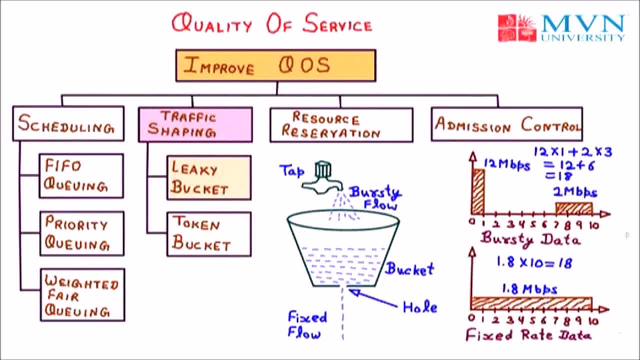 Can be converted Into Directly In 1. 8. MBPS And The data Can be set In The constant rate. If A bucket Has A small Hole At The bottom, 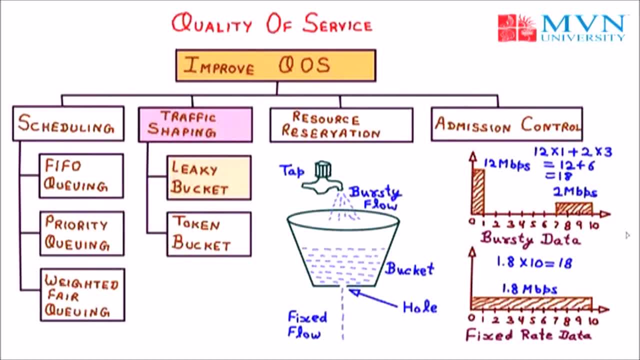 The water Leaks From The bucket At The constant rate, But The output Rate Remains Constant. Similarly, In Networking, A Technique Called Leaky bucket Can Smooth Out. 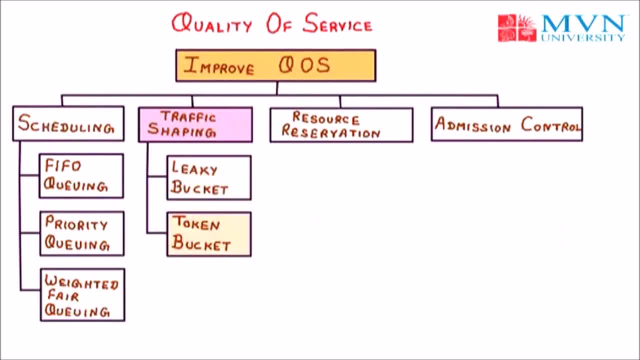 Bursty Traffic. So That's All About The leaky bucket. Next We Are Having The Token Bucket If The Host Has Bursty Data. The Leaky 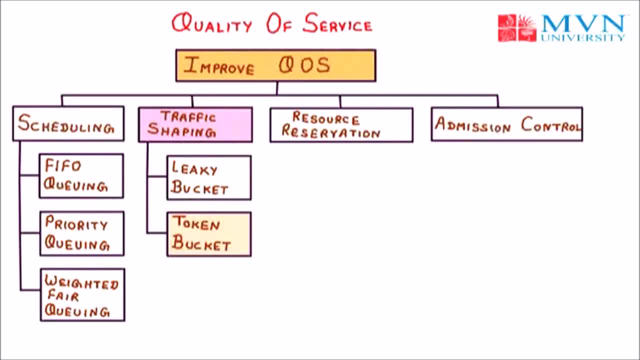 Bucket Allows Only An Average Rate. The Time When The Host Was Ideal Is Not Taken Into Account, So On. The System Sends N Tokens To. 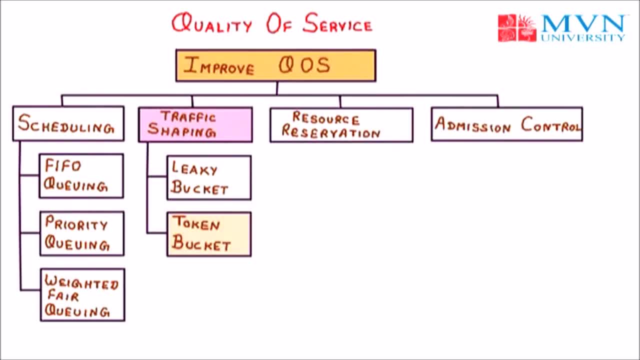 The Bucket. The System Removes One Token For Every Cell Of Data Sent. To Understand The Token Bucket, Let Us Take The Example. Suppose The Token. 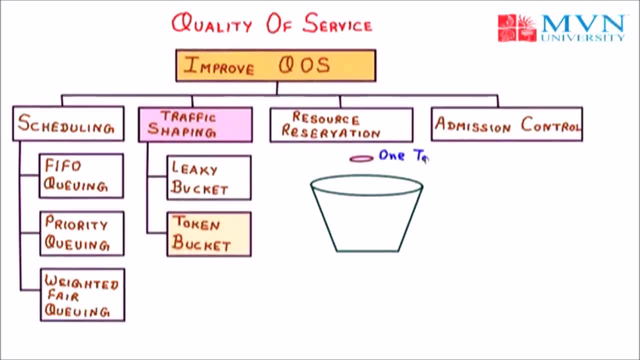 Is Generated, You Can Say That The One Token Is Added. Perfect, It Is That Trying. The Token Removed And Discarded For Self Transmitted Now. 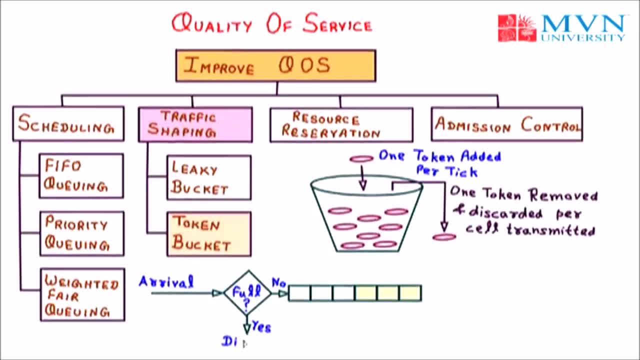 That Discarded Is Full. In That Case We Will Discard The Packet. Otherwise, We Send The Packet To The Queue And The Packet Will Be. 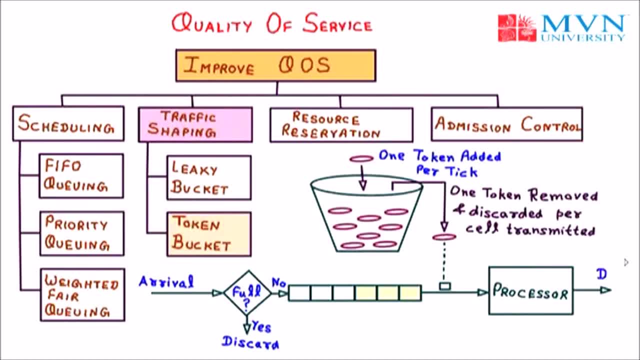 Added To The Token And The Token Packet. The Token Packet Can Easily Be Implemented With A Counter. The Token Is Initialized To Zero Each Time. 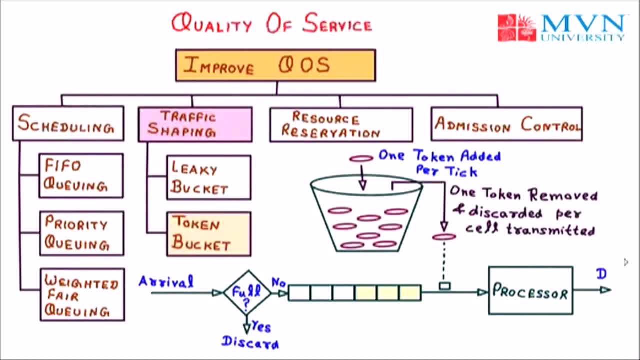 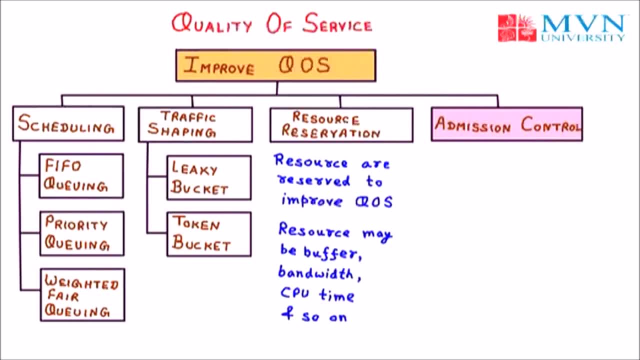 A Token Is Added, The Counter Is Incremented By The Token And The Packet Will Be Added To. The Packet Will Added To Zero The. 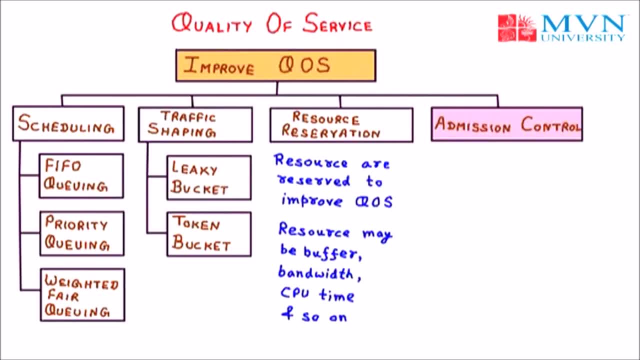 Token Is Added To Zero. The Token Is Incremented To Zero. The Packet Is Added To Zero. The Token And Token A Token Clock Is.